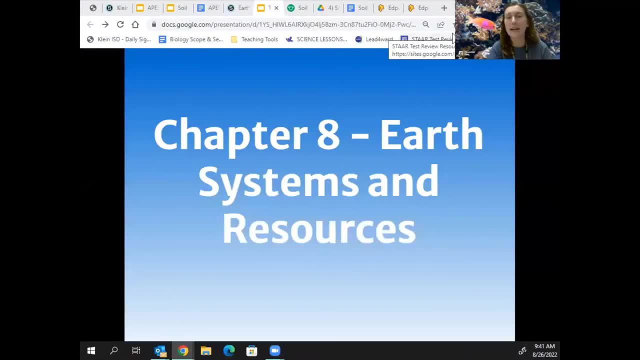 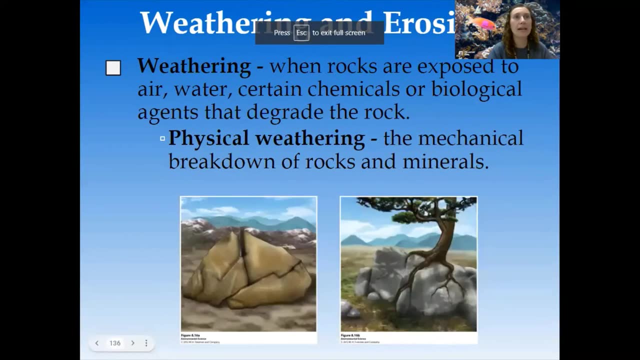 All right, good morning, good evening, good day, good night. I don't know what time of the day it is for you, but let's get into chapter eight: Earth System Station. Oops, I apologize, this isn't full screen. Okay, so so far we've talked a lot about the rock cycle. we've talked a lot 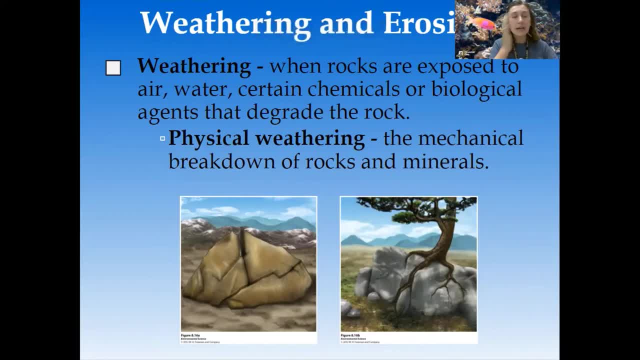 about plate tectonics- the ring of fire, of course. So now we're going to kind of transition to the third part of the geologic cycle, which is all about soil sciences. So we'll be talking first about weathering versus erosion, we'll get into soil formation and then we'll wrap up chapter. 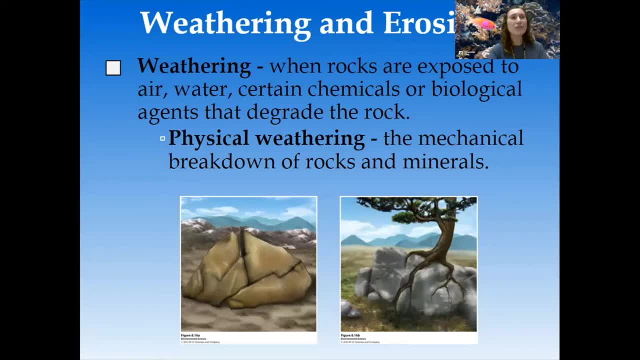 eight. Oh, also mining as well. All right, so let's first talk about weathering. So whenever I have some sort of rocks like the ones we learned about in the rock cycle, we can actually break down these rocks and expose them to elements. Weathering: the breaking mechanical down of rocks. 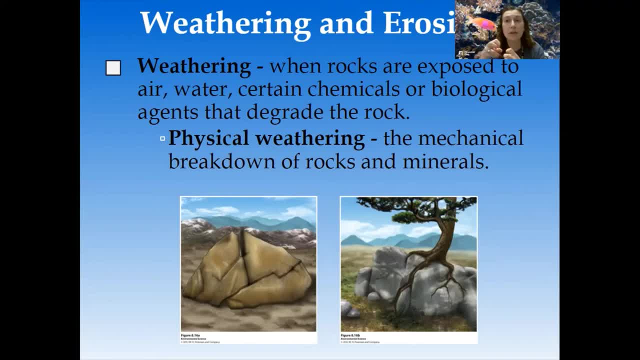 can occur via physical weathering: mechanically breaking it down, or chemicals, which we'll talk about next. In physical weathering- one we've got here- this is the exposure of rocks, usually to water. it can occur via wind, it can. 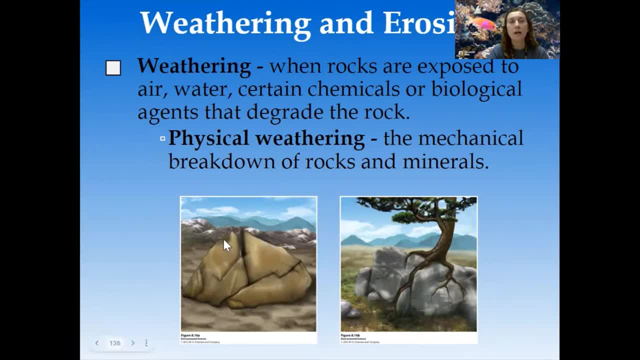 occur by plant roots- we'll talk about in just a second- But I mean, think about the Grand Canyon. that's an awesome example of a formation that has been weathered or broken down by the passage of water, pulling those particles, breaking down that as well. Mechanical weathering can also occur. 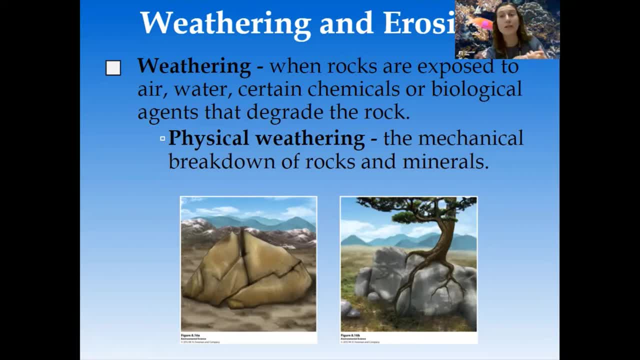 this physical weathering can also occur due to water in freeze-thaw cycles. So up north, where it gets cold and it actually snows- not Texas- if there's any water on the roads, that water can freeze, causing it to expand, because ice has a larger volume than liquid water. So when the ice expands and then thaws when it gets warm again and then expands when it's cold and then thaws when it's cold, that freeze-thaw cycle can also break down our roads. So up north, where it snows a lot, they actually have a lot of physical weathering of the roads there. 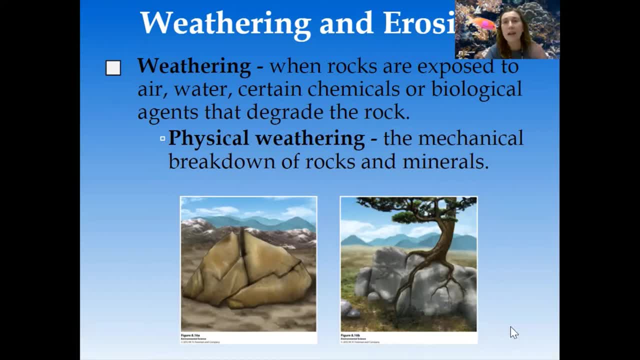 This can also occur via biological agents, via plants. I'm sure you have stubbed your toe a thousand times walking down the roads and then they're not going to be able to get out of the road. So this can also occur via biological agents. so via plants. I'm sure you have stubbed your toe a thousand times walking down the roads and then they're not going to get out of the road. 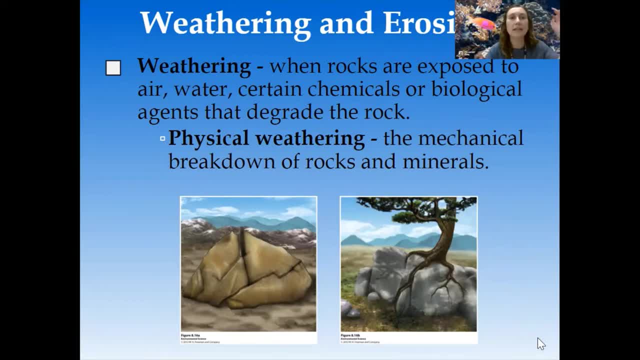 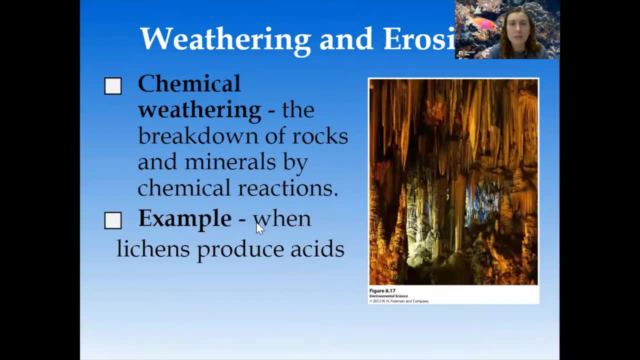 There are tree roots everywhere, so the tree roots can also, as they peer through and kind of work through. that's another form of physical weathering. The other form of weathering is chemical weathering. This is when we're actually looking at chemical reactions. So usually there is some sort of chemical, pH or different elements within the rocks themselves, depending on the metals, depending on the ions, whatever that composition of the rock is. 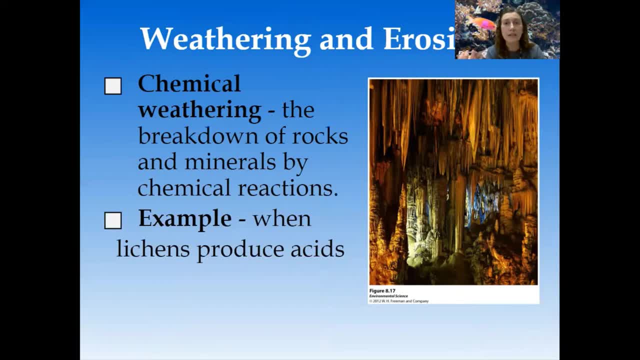 In chemistry you learn that solutions can be basic or acidic. So whatever my chemical composition is and the pH of any sort of chemical or liquid or fluid that is exposed to the rock, we can have a thousand different chemical reactions that can occur depending on the pHs and the chemicals either in the rock or what's being exposed to it. 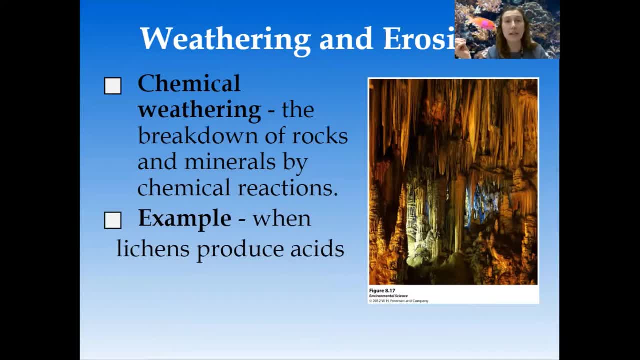 For example, sulfur dioxide forming sulfuric acid. So when we burn fossil fuels such as coal and oil, that's going to release sulfur into the atmosphere. Sulfur is going to form sulfur dioxide. We'll learn about that in our next unit. 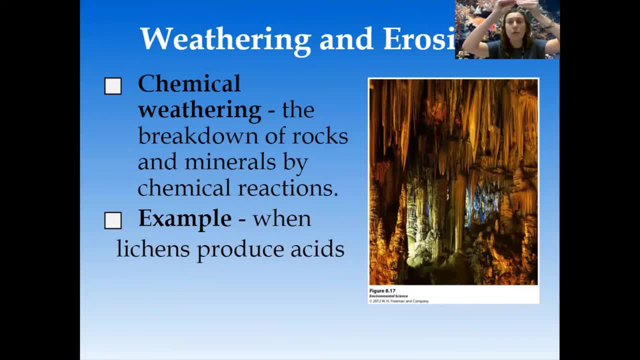 The sulfur dioxide in the atmosphere can then combine with water vapor, forming sulfuric acid. Sulfuric acid is one of our two forms of acid rain. We'll learn about this later on this semester when we get air pollution- but that acid rain falls down and can break down different stones- things such as gravestones or statues. 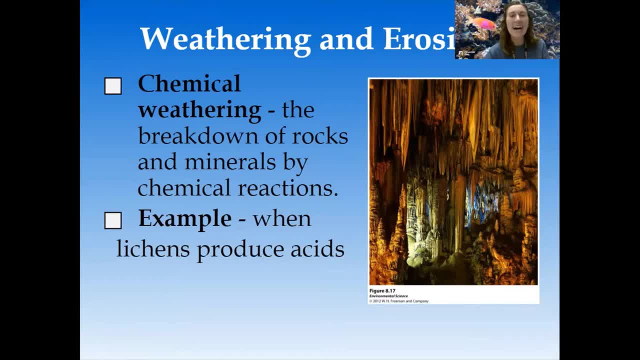 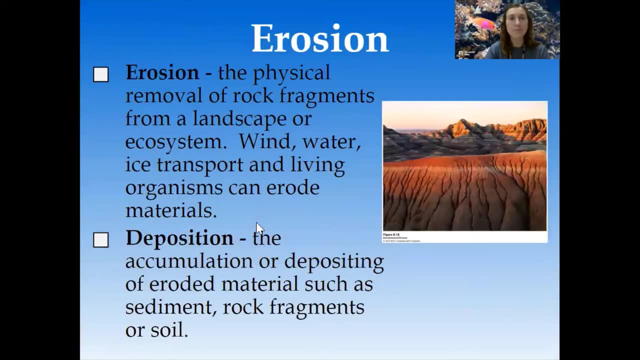 I feel like my brain is not working, so thank you for hanging in there with me. But that is one example of chemical weathering. When I'm actually having some sort of chemical applying itself to the rocks and chemically breaking it down, I oftentimes see weathering versus erosion getting mixed up. 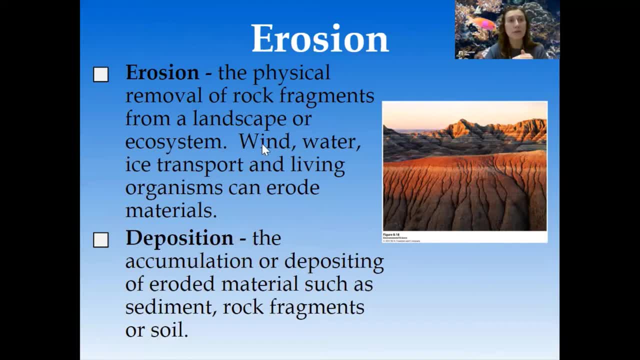 So I wanted to take just a little bit of time to talk about weathering versus erosion. So when we're talking about weathering, that's the physical or chemical breaking down of the rocks. Once I break down those rocks via weathering, erosion kicks in. 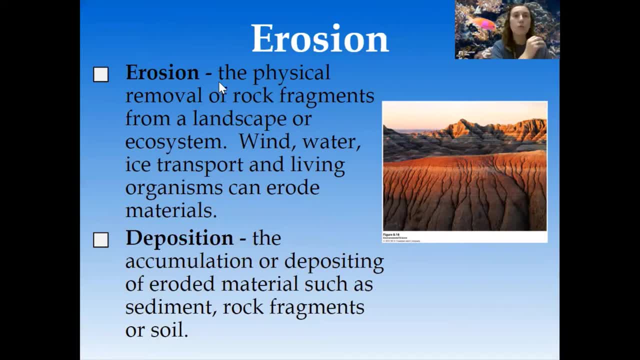 Erosion is the movement of those broken down rock particles. So I've weathered it down. Maybe it's rained, Maybe I've got some acid rain. We're picking apart the rock. Once I have these loose particles, then if there's wind or if there's water or animals transporting those particles from one place to another, that is going to be erosion. 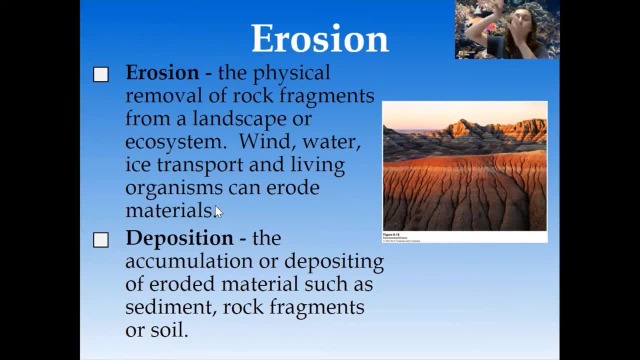 Erosion can also happen via gravity as well. So if I have a rock formation, a piece of rock falls off, that's going to also travel via gravity. Maybe it's going down the hill, So I've had the weathering that broke it down- erosion that moves it. 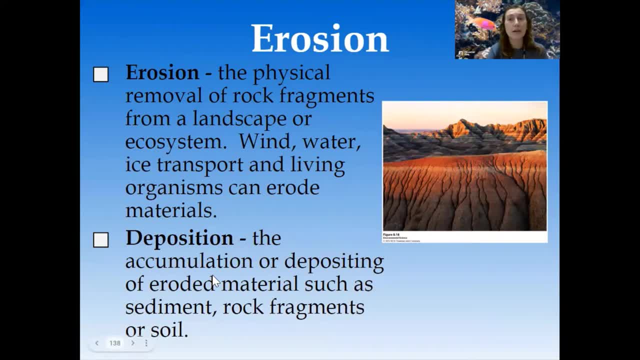 Finally, I'm going to have deposition. I'm depositing or putting down the rock somewhere. So wherever those rocks eventually settle onto is going to be the process of deposition. We're going to be talking a lot about this at the end of this Ed Puzzle, when we get into mining. 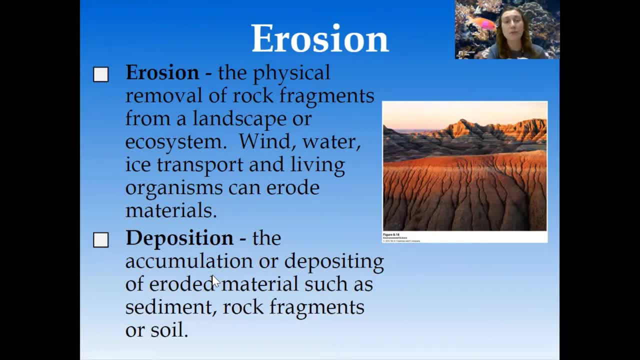 where, when we're actually breaking down rocks in order to mine for different materials, that could be a problem If we're exposing to lots of different chemicals in those rocks And then those chemicals on the rocks get deposited further down the stream in our ecosystems. 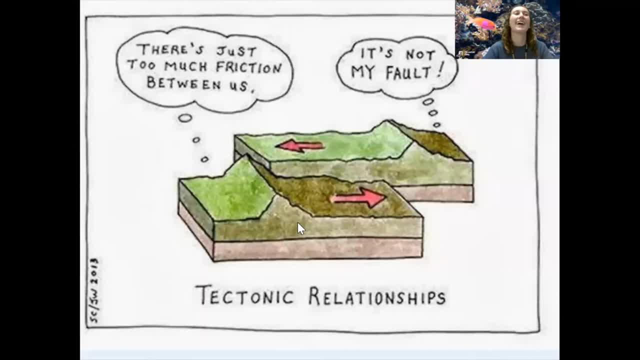 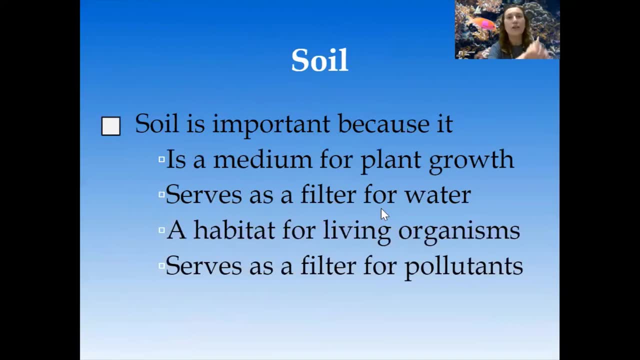 But we've got to break things up with a joke. So there's just too much friction between us. It's not my fault, Ha ha ha. A ton of relationships, Okay, So soil is one of the most important resources that we have in our world. 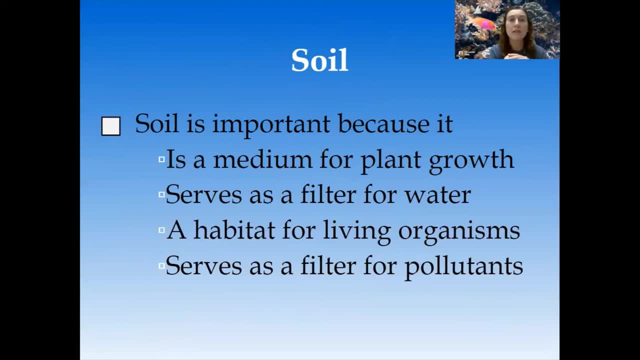 The formation of soil and soil properties is going to be the third part of the soil, Third part of the geologic cycle, In concert with tectonic plates and also the rock cycle. So tectonic plates, rock cycle you've learned about with your earth system stations. 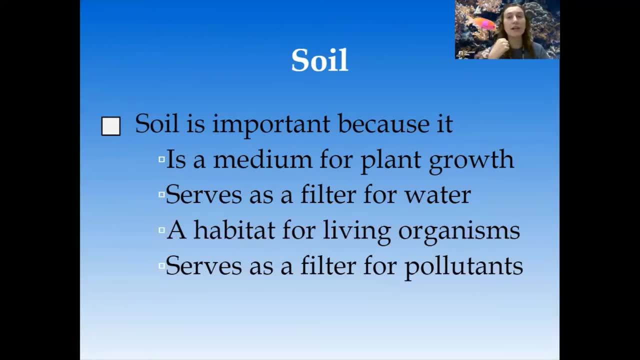 Now we're bringing in soil formation. Like we said during apes trivia, soil takes an incredibly long time to form, but it's incredibly important for us. It's going to have some geologic rock components and it's also going to have some organic components. 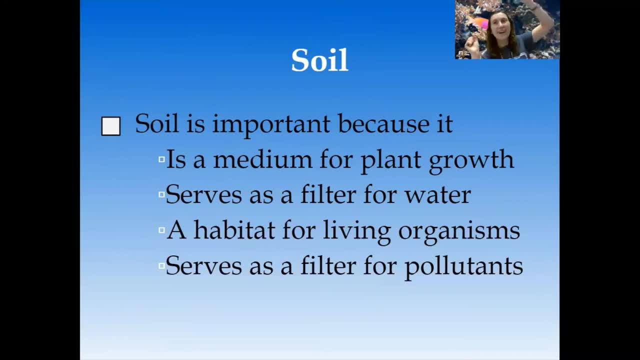 So we're bringing in some life Finally- life in environmental science- But we'll talk about how that actually happens. Okay, Does a lot of good things. Look at all those good things it does. I'm not going to read all of them, but you can read them. 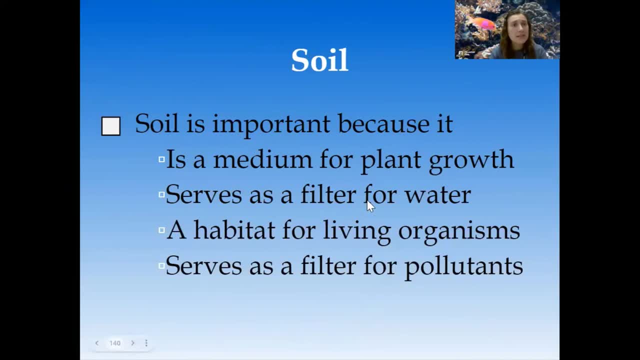 But it really does filter a lot of things. It's going to create habitats and it's going to help us out, especially if we ever have any chemicals, So those pollutants aren't actually getting into what's our aquifers underneath the soil or groundwater reserves. 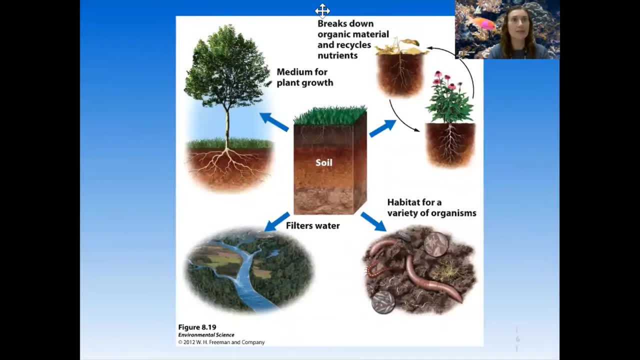 Okay, Look at all the great things it does. Anyways, this is just another graphic kind of demonstrating. I would maybe make sure you know all the good things that soil does for our world. Okay, I'm not going to read that one out loud. 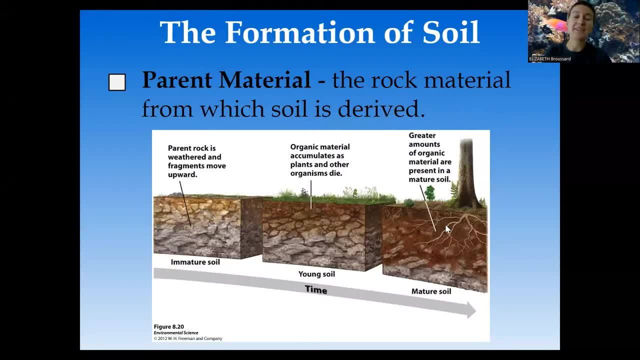 Okay, Sorry, I had to restart that because I got a little laughy there. So let's talk about the formation of soil. We've said so far that soil is incredibly important for a lot of different reasons, And at the very beginning of the year we learned that it takes anywhere from hundreds of years to thousands of years in order for that soil to develop. 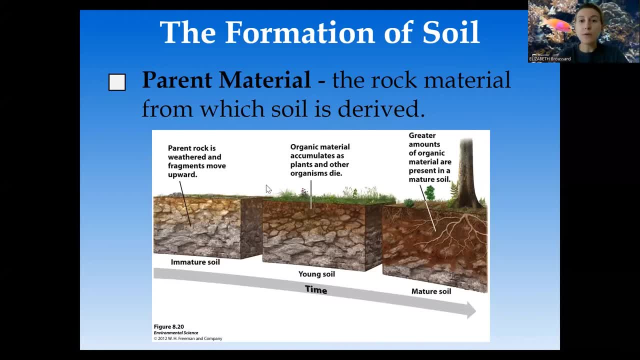 So let's talk about what exactly is going on in that process When we're forming soil. Soil, essentially, is going to start from weathered rocks, So we call this the parent material, And the parent material over many, many years is going to be weathered and broken down into smaller and smaller pieces. 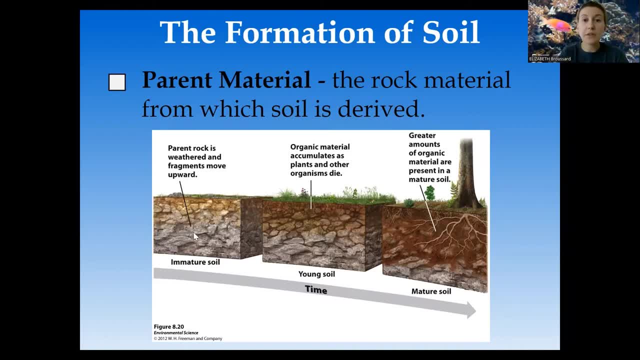 As the parent rock. these minerals are weathered down. it's going to intermingle or mix with organic material from the surface. This organic material can be decomposing organisms. This could be like dead twigs. This could be lots of beetles. 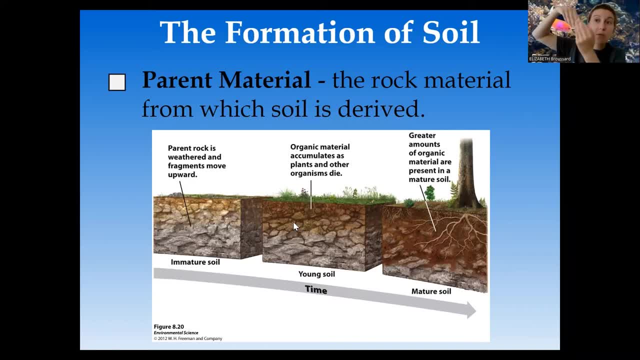 As the organic material, though, begins to mix with the weathered rock. that's how I'm going to start making soil. We call this that young soil. Over even more years, and even more and more time, we get more and more organic material. 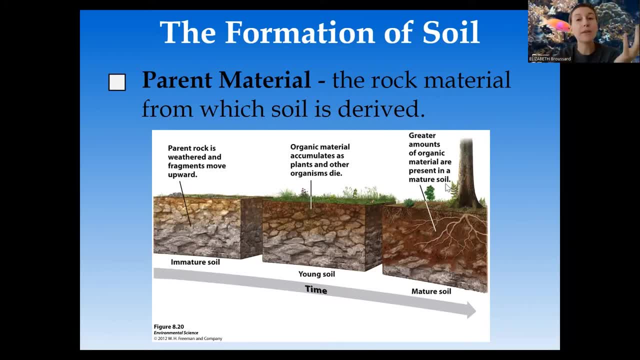 And that's how we're starting to create our soil. So the greater amount of organic material mixed in with these minerals- it's going to tell me how profitable or how fruitful that soil is. The very mature soil is going to have a lot more organic material than very young soil. 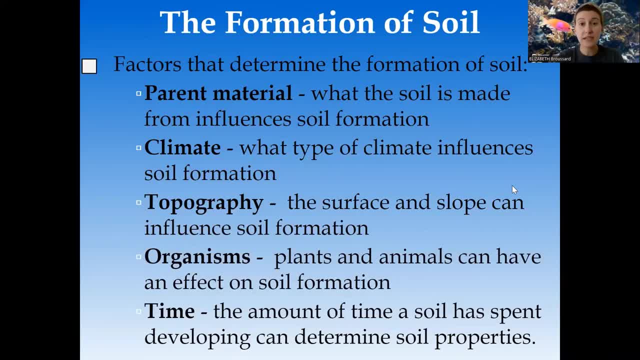 All right, A couple of things. I'm not going to go into each of these in detail, but these are some five factors you should be familiar with that's going to tell me about how fast or how this process of forming the soil is going to go down. 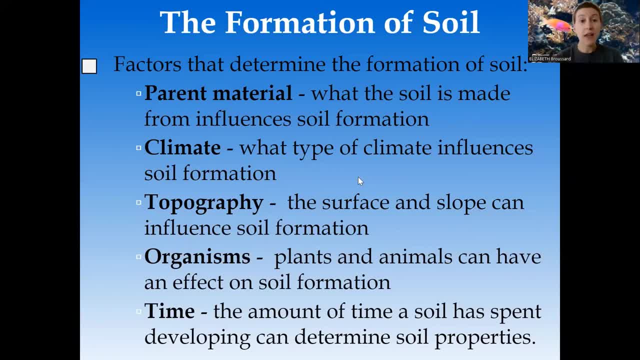 So, depending on what the soil is made out of, the climate that we're in, what is the weather like, what are the temperatures like, what is the surface, the organisms available, how much time it has spent, all these factors are going to tell me how good my soil is going to be and how long that soil is going to take to actually be produced. 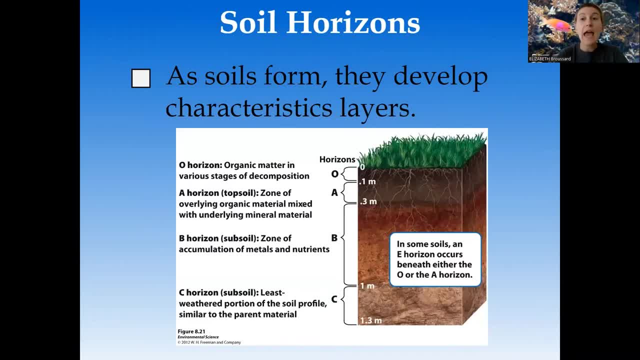 All right, All right. So what is the soil going to be created? As my soil is creating, it's going to develop into four distinct layers known as horizons. These are our soil horizons. I'll have you guys come up with an acronym to help you remember, because it is like ABC. 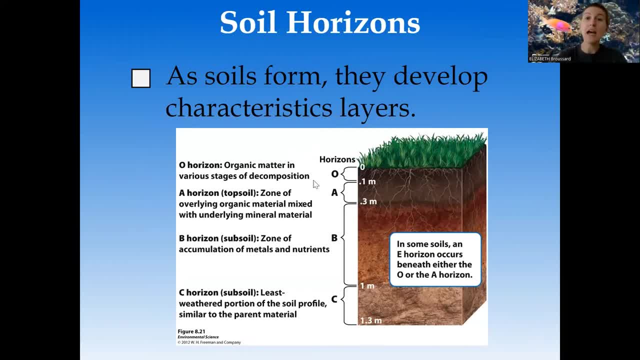 That makes sense, But the fact that O is at the top, I'm like what? But these layers can have varying thicknesses as the soil is continuously developing along that development timeline. So let's talk about each of these layers- the O, A, B, C horizon- in detail. 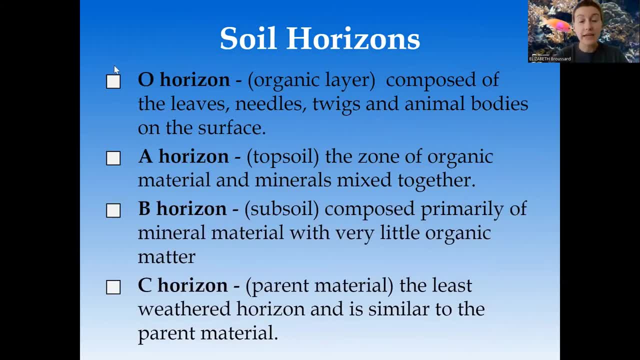 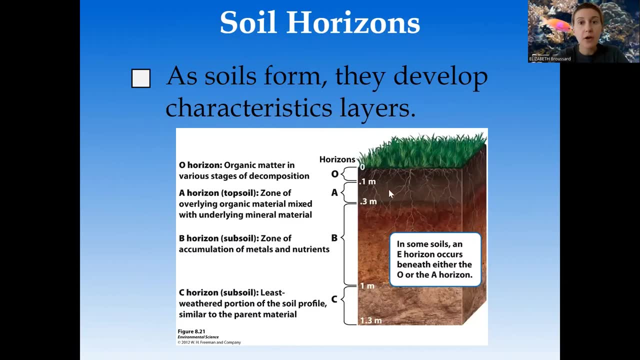 The O horizon stands for the organic layer. O is for organic, That's the way you can remember it. This is my very, very top layer. So if we're looking at it over here, my O horizon is going to have the most living materials. 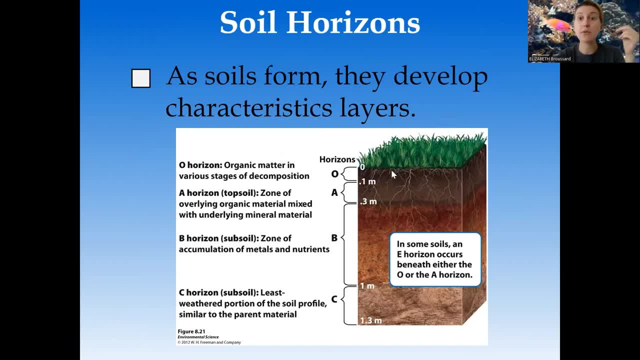 This is going to be where a lot of my bacterial is: my beetles. This is going to be where primarily my roots are, from my different plants, Lawn clippings- all of this is going to be part of my organic or my living layer. 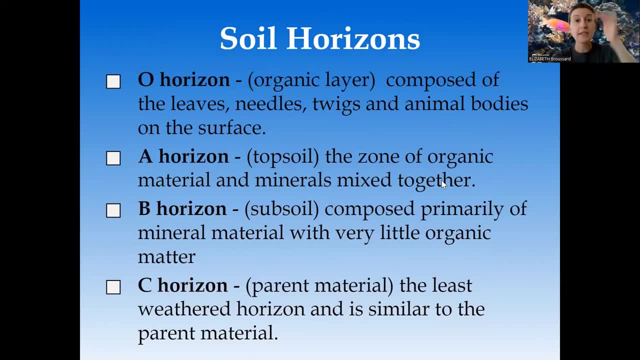 Also decomposing organisms are going to be found in there. As I move down now I get into the proper topsoil. This is my soil, proper Compared to the A, B and C horizon. excuse me, compared to the B and C horizon. 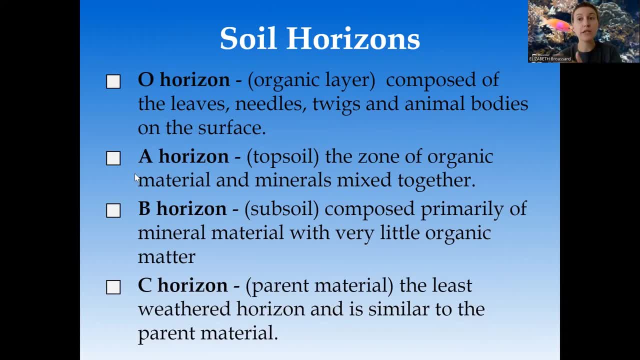 the A horizon is going to have the most organic ratio compared to how many minerals, So greater amount of organic material, less actual minerals or rock fragments coming from that bedrock at the very bottom. We call this also this topsoil. It's the most nutritious. 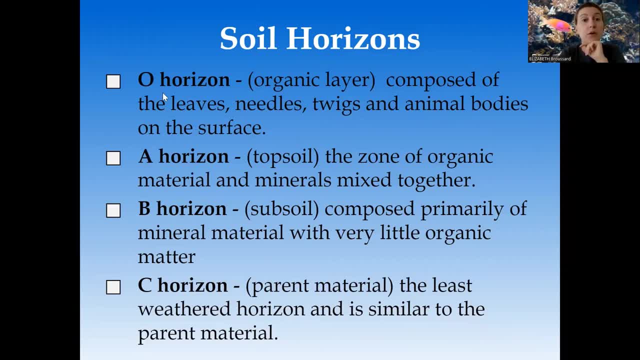 It's the most fruitful soil compared to, Compared to the O horizon. My B horizon is kind of- I'll talk about the C in just a second- But the B horizon is kind of like, I would say, the child or the mixture of the A horizon and the C horizon. 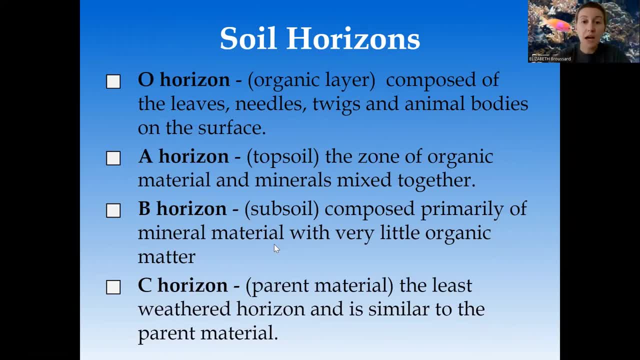 We call this the subsoil because it's right below my topsoil. My subsoil is going to have if the O, if the A horizon had more organic compared to minerals. B horizon is going to be the opposite: It's going to have more minerals compared to C. 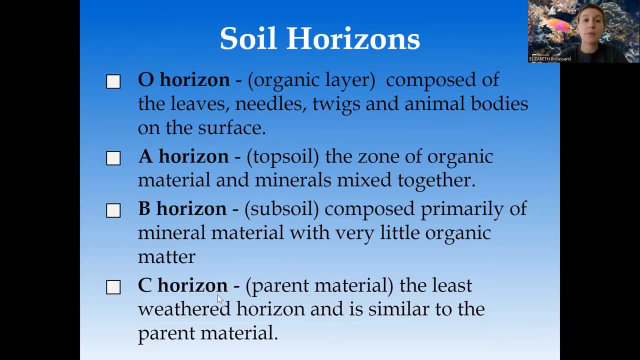 It's going to have more minerals compared to how much biological or organic material in there. So primarily minerals with a little bit of organic. Finally, I get to that C horizon. The C horizon is going to be that parent material. This is essentially the bedrock. 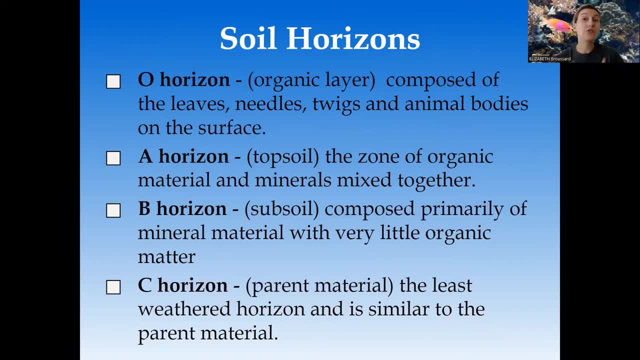 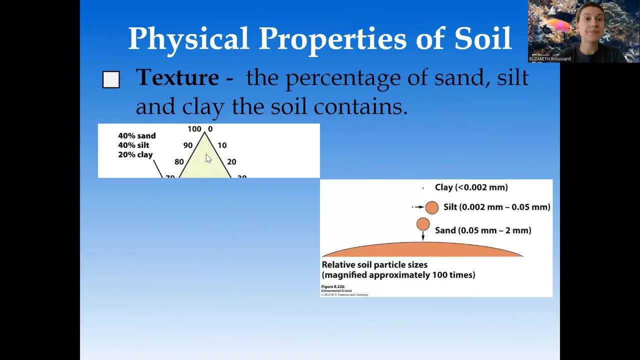 So it's primarily rock that's starting to break down and eventually will become the B and then the A horizon as it moves upwards closer to the surface. All right, I would be remiss if I didn't talk about the physical properties of soil. 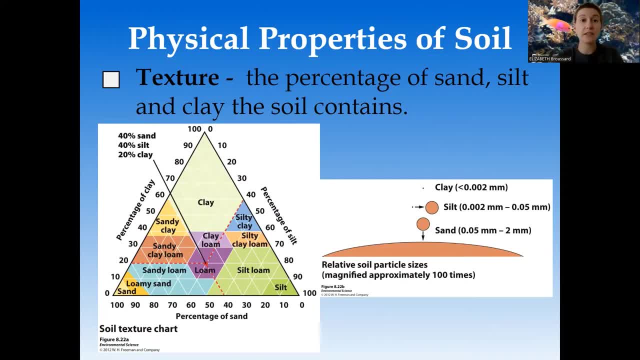 We're getting into our soil labs. You're going to become very familiar with these two graphics here. The texture is what we refer to as in a soil sample, how much sand, silt and clay the soil contains. Sand, silt, clay are the three major components that makes up soil. 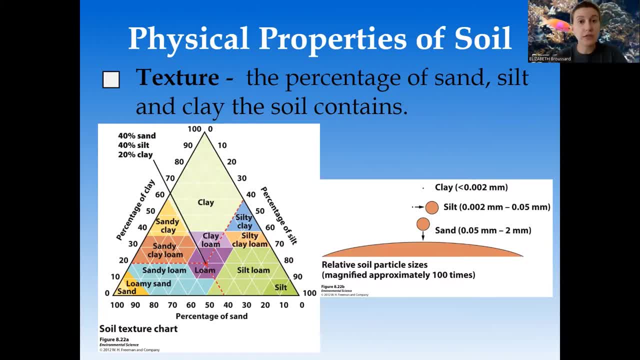 And all soils have all three of these in varying degrees, Depending on what those ratios are- how much sand, how much silt and how much clay. it's going to tell me what kind of soil I have. Looking on the right-hand side, we can kind of see it as reference. 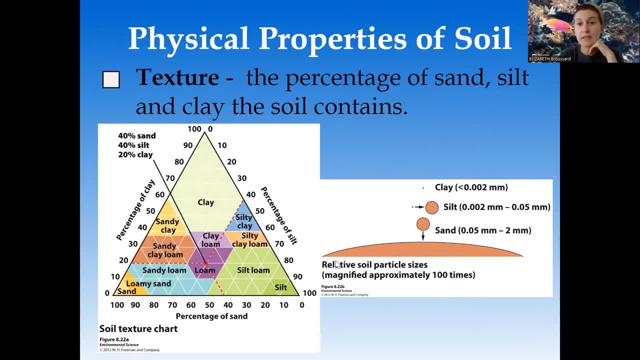 How big a particle of sand is. that's this giant one here compared to a particle of silt, compared to a particle of clay. So sand is my largest ones, silt my medium size, and clay is going to be the tiniest one. 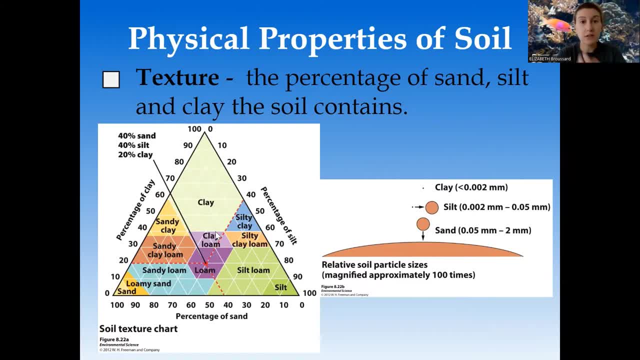 We'll talk about that more in a second. We're also going to learn in just a second how to read this cool graphic. This is actually one of my favorite graphics, called Soil Triangle. You'll need to be familiar with both of these as we get closer to our quiz and our test. 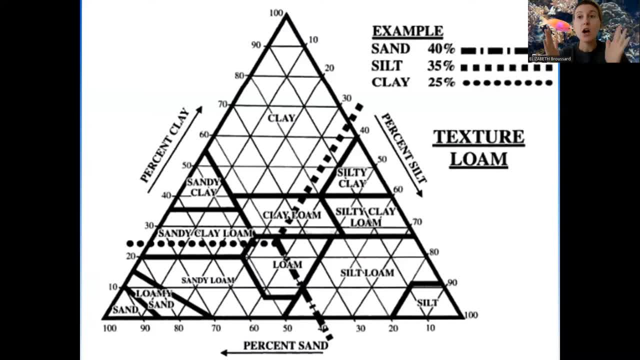 All right, Let's look at the soil triangle first. So as we look at the soil triangle, as I said, all soils have a percentage of sand, silt and clay. Depending on those percentages of their compositions, that's going to tell me what kind of soil it is. 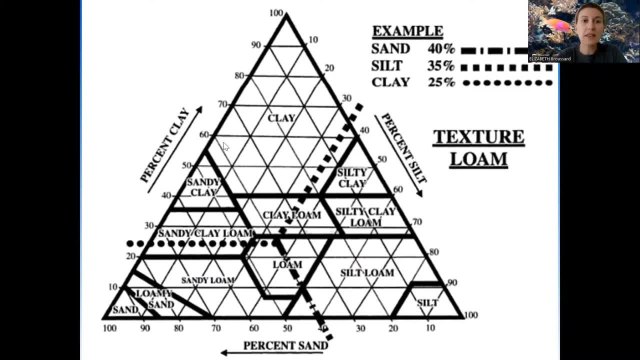 So I want you to pay attention to something. Let's say, on the left-hand side, I'm looking at percent clay. You see how there's an arrow going upwards. The arrow is pointing up, up up. That arrow pointing upwards tells me when I'm looking at a particular percentage. I'm going to use the upward line. 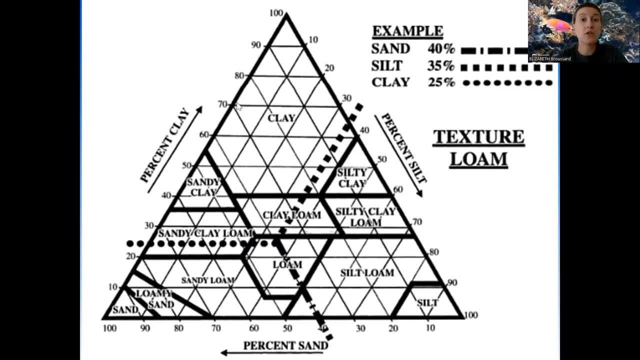 So out of 70%, let's say, I have two lines coming out of 70%. I need to pay attention to the top line because my percent clay arrow is pointing upwards. Same thing percent silt The arrow is pointing down. If I looked at the 20%, there's two lines going out. 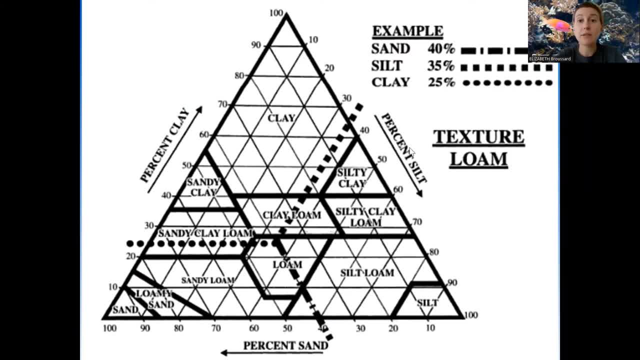 But I'm going to look at the arrow or the line that's going down, because my percent silt arrow says point down, point down. So let's look at this example: Sand is 40%, silt 35, and clay 25.. 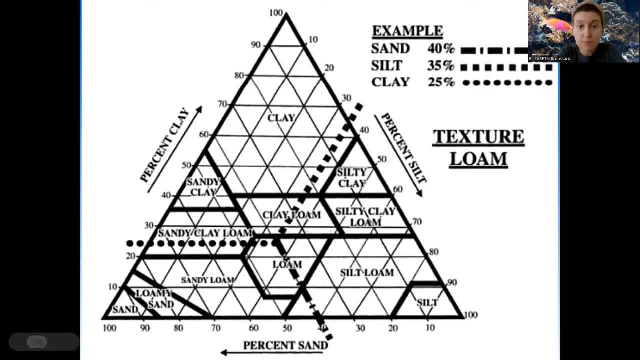 So I'm going to look for sand 40%. I'm going to go down this percent sand at the bottom, Find the 40. My percent sand arrow is pointing. I don't know if my hand's going the right way, but it's pointing to the left. 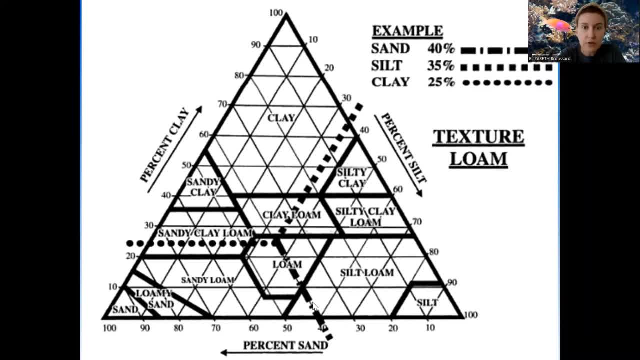 So I'm going to use the leftmost line. I'm going to go ahead and draw a line right there. Okay, Silt is 35%. Again, I'm going to go to the percent silt over here. 35 is right in between 30 and 40. 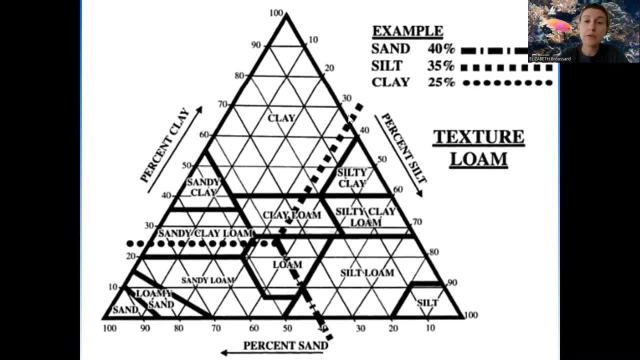 My arrow is pointing down. I need to use the bottom line or the bottom direction. That is going to go ahead and intersect with my percent silt. But just to make sure, percent clay is 25%. It's about halfway between 20 and 30.. 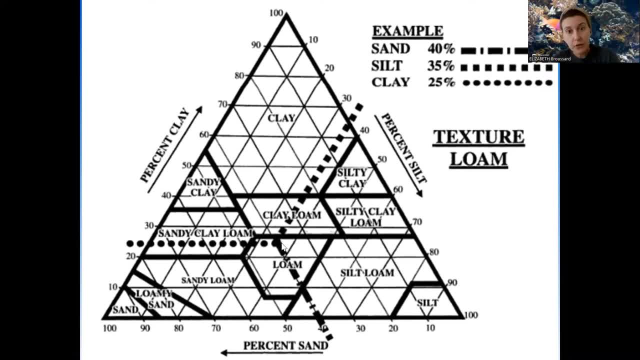 Arrow is pointing up. I want to use that utmost line. Those three lines intersect and I find out that my soil sample with these particular parameters is alone. That's the type of identity that my soil is. We're going to practice this. 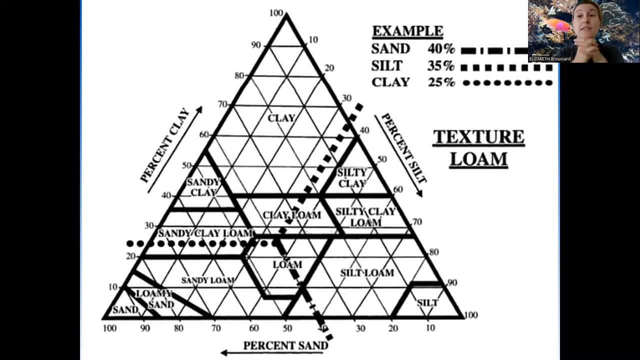 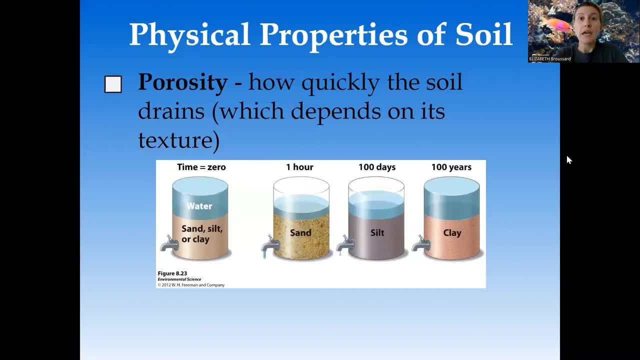 You're going to do this at least three, if not five, times in class, You'll become very familiar. But just kind of introducing you guys to our lovely soil sample. Additionally, when I'm thinking about how much sand, silt and clay is the composition of my soil sample. 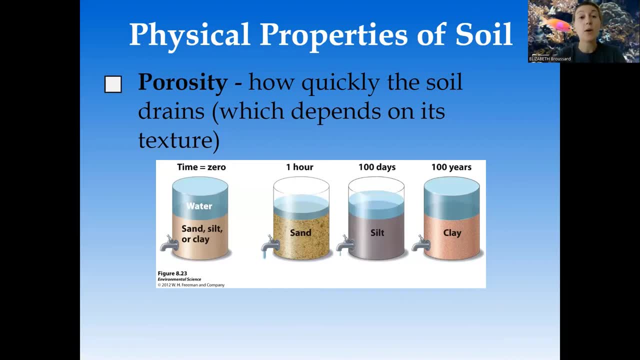 that's going to also affect two properties called porosity and permeability. Porosity is looking at the actual pore sizes or open spaces in between the particles in my soil sample. It's going to affect permeability- the ability for water to flow through the sample. 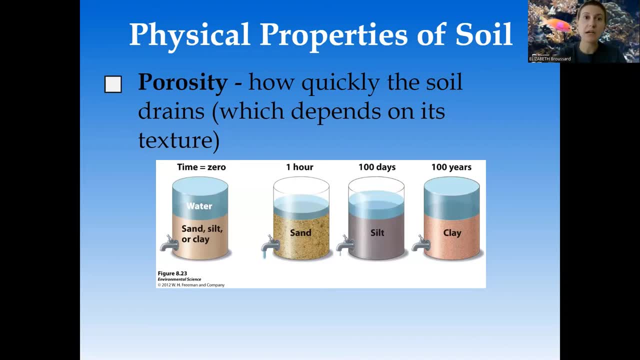 We'll talk more about this in class. I have a nice diagram for you guys. So sand, silt and clay. Sand is my largest particles. If I have very large particles, when those two, when all those large particles stack on each other, I'm going to have a lot of open space in between each one. 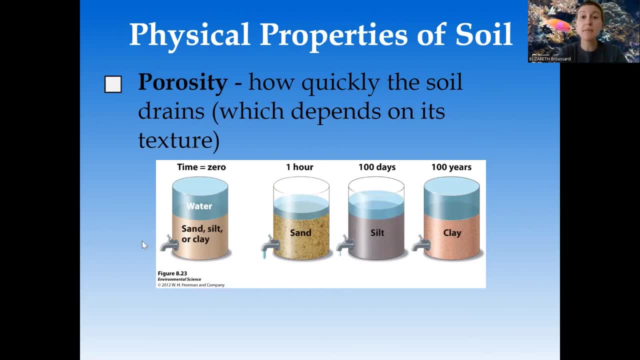 Those big open cracks or big open spaces means that my sample is very porous. A lot of water is going to be able to flow through it. because of those big porous sides It's very permeable. So let's say in this example, sand, this would only take about an hour to flow this amount of water. 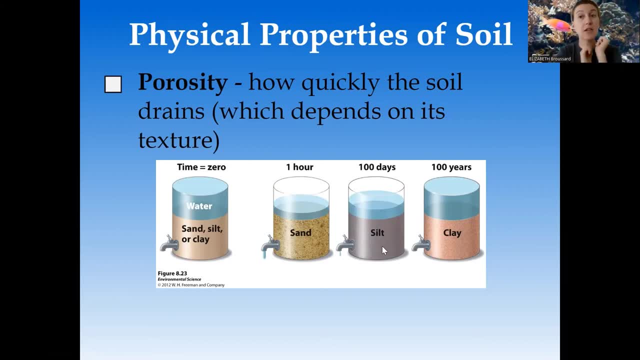 Silt is going to be my medium-sized particles. It's a little bit smaller than my sand, which means also the porous sizes are smaller too. If my porous sizes are smaller, less water is going to be able to flow through, which means it's going to take a longer time for water to flow through because it's less porous, less permeable. 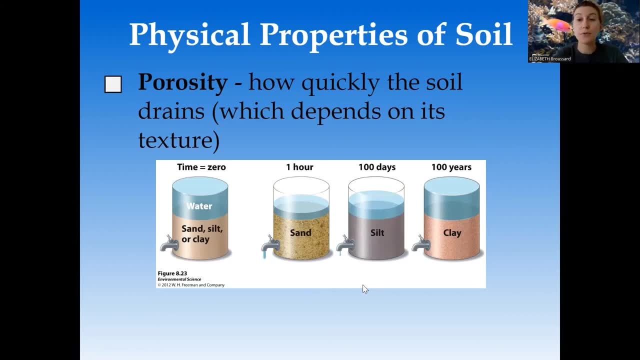 So maybe this would take 100 days for this amount of water to flow through. Clay is my smallest, tiniest particles. Think about if you've ever held like molding clay in your hand. It's super silky, It's super soft, It's not very coarse and brittle like sand is. 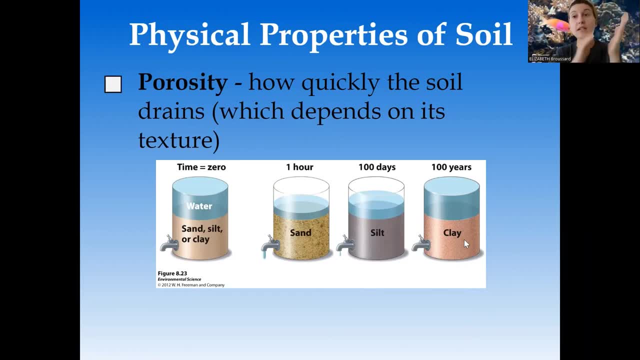 So clay is the tiniest particles, And because clay is the tiniest particles there's the least amount of space. It's very difficult for water to go through just pure clay, And so this is the least porous, least permeable type of soil composition. or 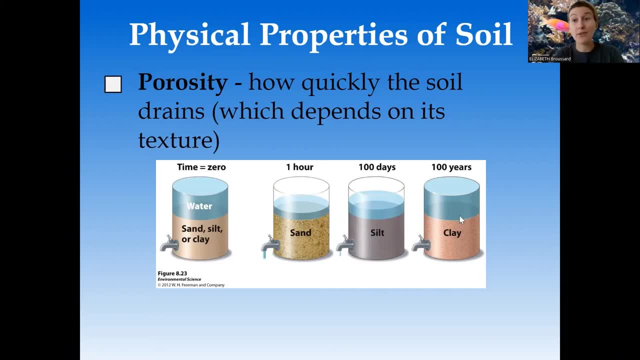 component. So this would take 100 years for that water to go through, because it's really not trickling through. It's good to know these different properties, especially as we're thinking about when we talk about water pollution. we'll be talking about landfills. 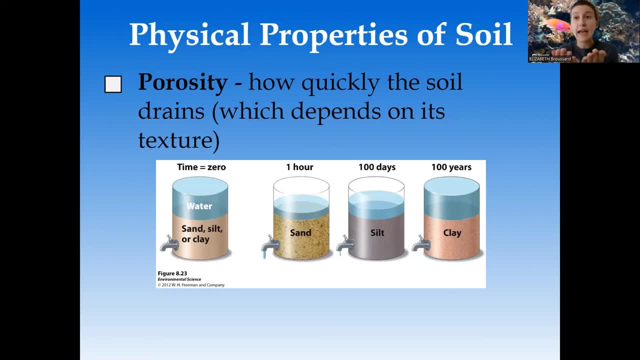 Landfills are usually lined with clay, and they line landfills with clay because they don't want all that toxic waste in the landfill to seep down out of the landfill and into my groundwater reserves, known as aquifers. I want to keep all that stuff. 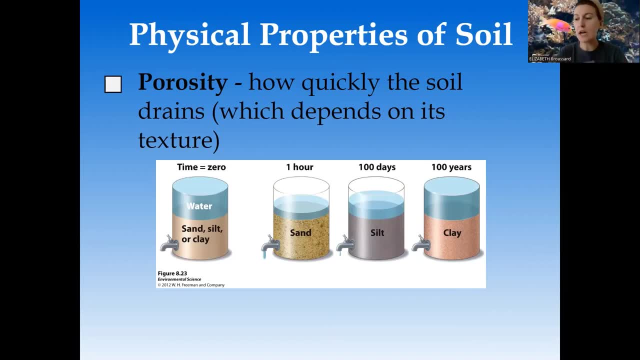 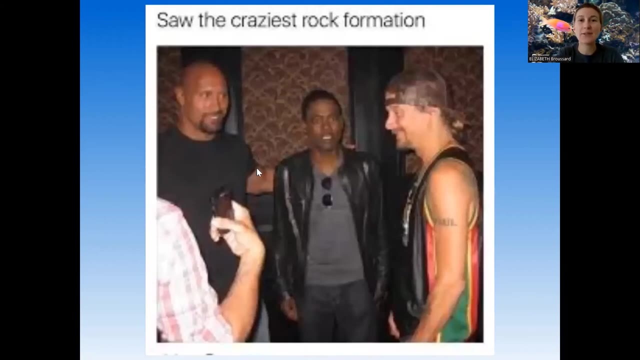 packed in place, which is why a lot of times, landfills, manure lagoons, a lot of these are going to be filled with clay or lined with clay so that the water or the toxic waste doesn't actually seep through. All right, last joke. I swear This is the last joke. I just thought it was funny, Haha. Dwayne's a rock, Queen's a rock, kid's a rock. 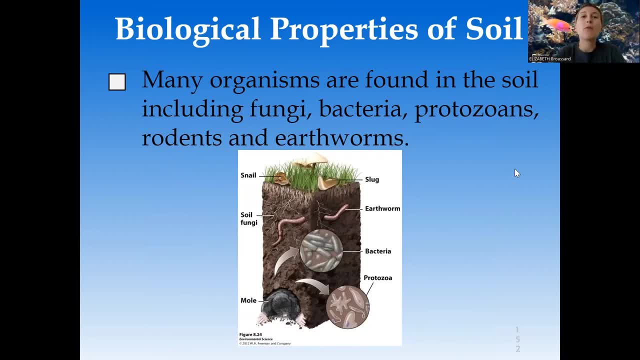 Okay, we're almost done. Biological properties of soil, When we're actually thinking about the living parts. earlier we were just talking about the physical properties, now we're talking about the living biological properties of soil. This is essentially. we're looking at what is living in my soils compared to the non-living components, such as the minerals or the rock. 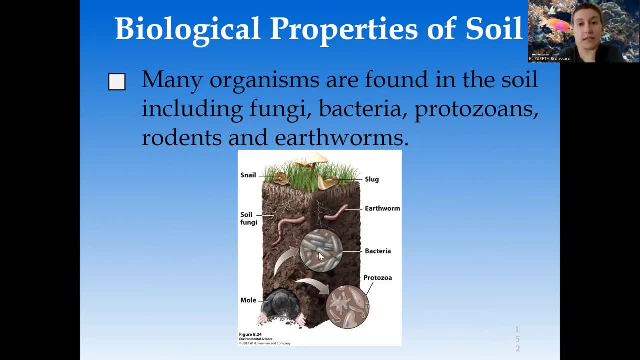 compositions of it. One key thing I'm going to point out to you guys is going to be our bacteria. These are my microorganisms. They are living because it is made up of cells. Bacteria have cells. When we get in like two, three weeks or so, when we get into nitrogen cycle, we'll talk about nitrogen fixation. We'll talk about nitrification and denitrification. 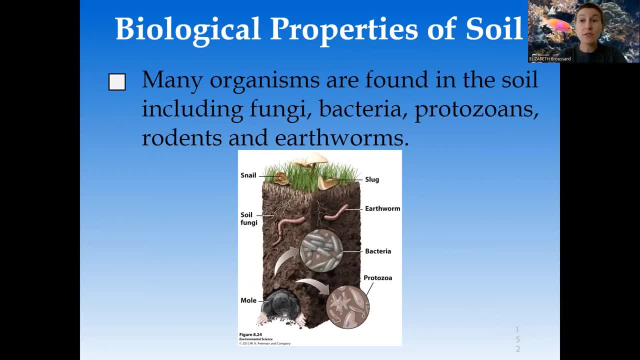 And that's a huge critical part of my nitrogen cycle, circling those nitrogen elements throughout my entire world and my biospheres. And bacteria is a key player in the nitrogen cycle. So all the wonderful living things that live in my soils are incredibly important, not just for the health of the soil and the nutrients in the soil itself, but also my entire biosphere. Everything is interconnected in this class And that's why I love it. I mean, everything just works. 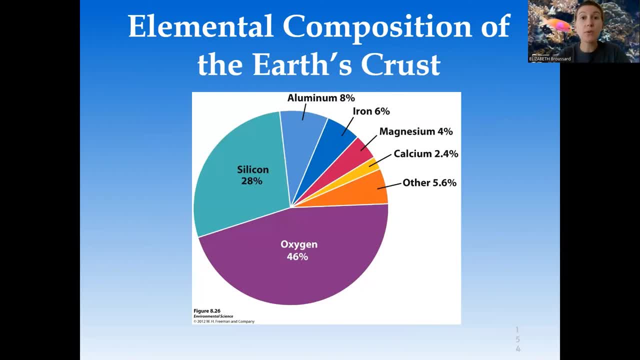 All right, last, last concept: We're going to talk a little bit About what's going on in the elements of composition of the Earth's crust. We'll talk about mining and then we're done after that. So this pie chart is just kind of giving us an overall view. 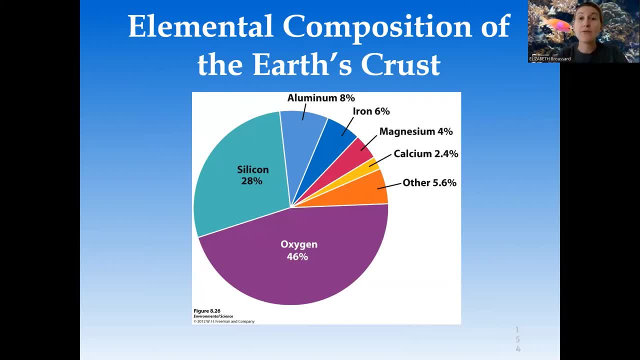 Excuse me, I almost choked Of all the different elements that we can find in Earth's crust. Really, in particular, we're going to be looking at these kind of over here on the right hand side. These are going to be my metals. 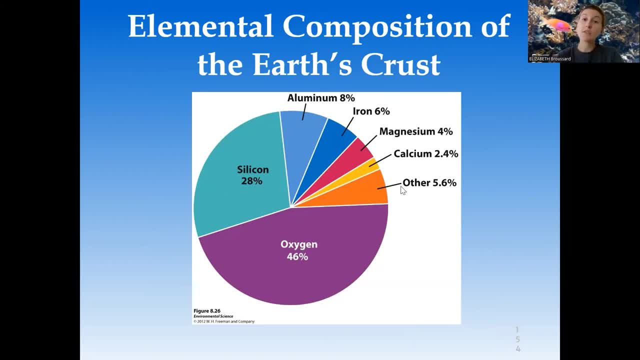 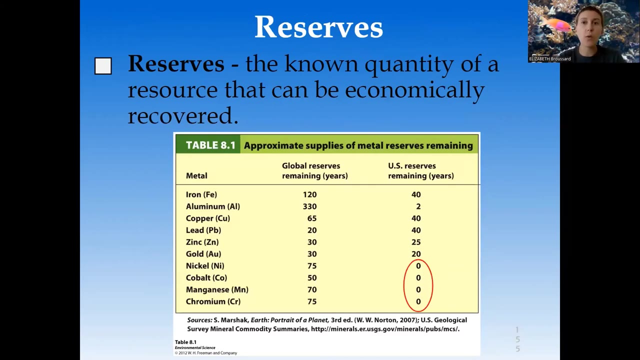 And the metals are going to be very precious resources that will actually get into mining in order to extract these resources, these minerals and these ores, from my Earth. That way I can actually utilize them in, usually in industrial processes. Reserves is going to be the known quantity of a resource that can be actually recovered for a different location. 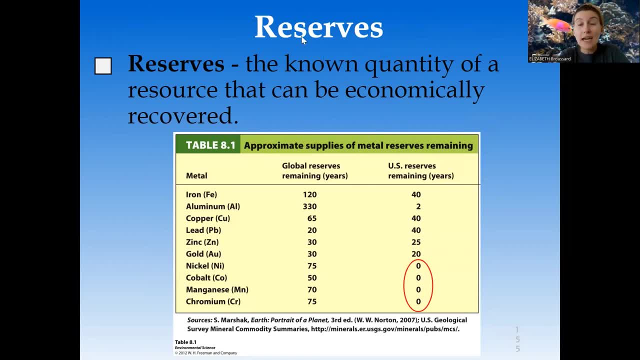 The reserves. I want to point out that this is the known quantity. A lot of times land is going to be privately owned by different corporations and they don't always share that information about what their reserves are like. So really, this information here, This is approximate. 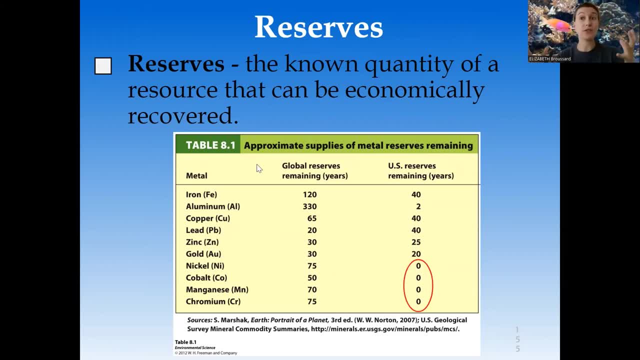 Because one we don't know as things are being reformed, Like how much there is at a given moment in time, but also because we don't have all the complete information right. We only have the publicly known information. If anything is privately owned, not all. 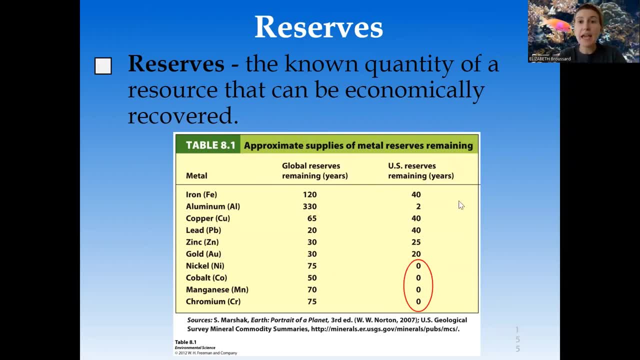 We don't always know what that information is. The reserves are going to be? how many remaining years? So if I continue to mine at the rate, I am taking into consideration how much time it takes for a lot of these to actually form and recycle. 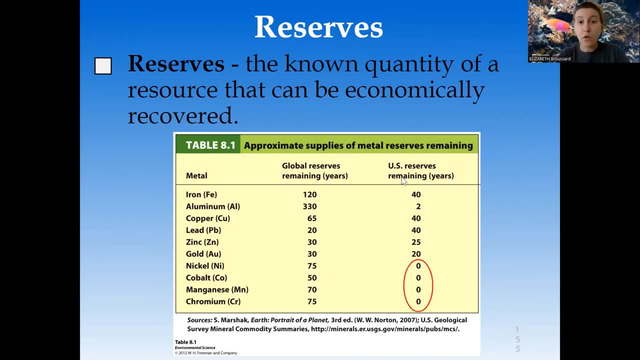 This is the remaining years that we have left of each of these, So globally we're doing pretty good, But a lot of reserves, at least in 2007,. the United States actually ran out, So things like nickel, cobalt, manganese and chromium. 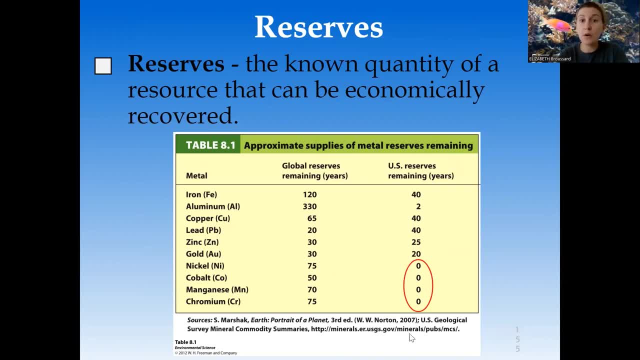 We actually have to import from other countries because the United States has actually run out. And I'm actually very curious and we only had two remaining years as of 2007.. I'm curious to know if we even have aluminum anymore On site. 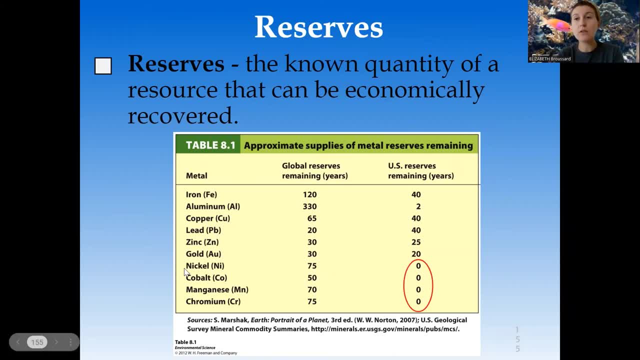 So a lot of these we still have to import. You probably have heard like with nickel our coin, like our handling our money coin. Those compositions have changed over time because a lot of these ores and these metals are actually becoming more and more rare. 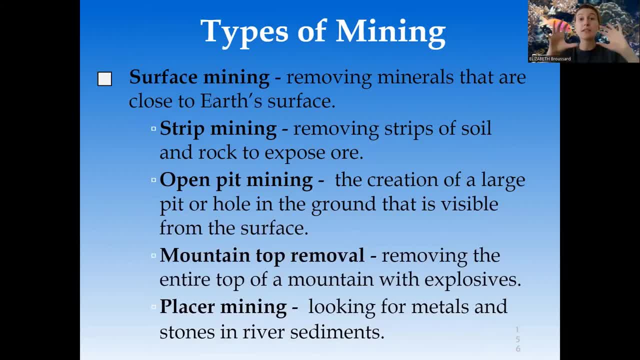 We have two main types of mining, or the processes to actually remove and take out these metals and extract them from our Earth. We have surface mining and subsurface mining. There is four types of surface mining, But thank God There's only one: subsurface mining- surface mining. 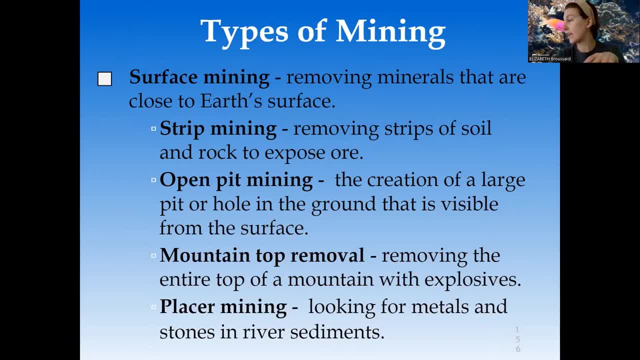 The differences between these is essentially what is my overall process, and I actually have my textbook here. I highly recommend going to page 227.. Oh, are you gonna be able to see it? No, you cannot. Okay. Anyways, 227 in the textbook has a wonderful diagram that goes over each of these strip mining. 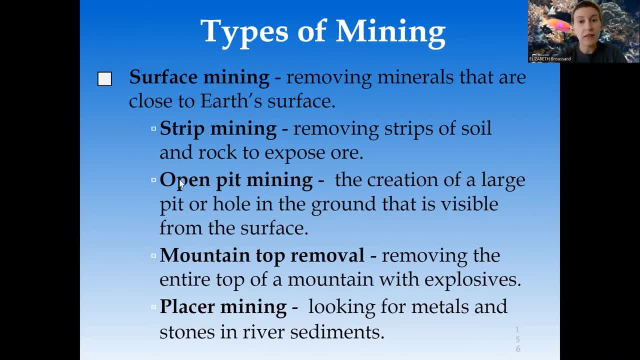 It's a lot of these. I'm not going to go into super big detail because they- a lot of them- are kind of self-explanatory, like open pit: We're digging a big pit, cluster mining We did a lot for during the gold rush. 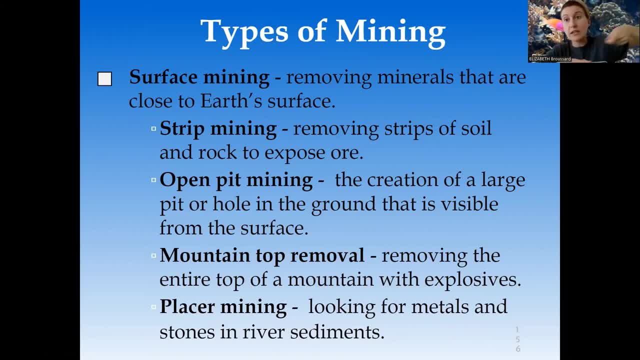 That's whenever you take the, the pans and you go into a riverbed and you're looking for it in the sediment. So we were shaking out those pants, panning for gold. you know, back in the gold rush That's our plaster mining. but I do recommend page 227 be really helpful. 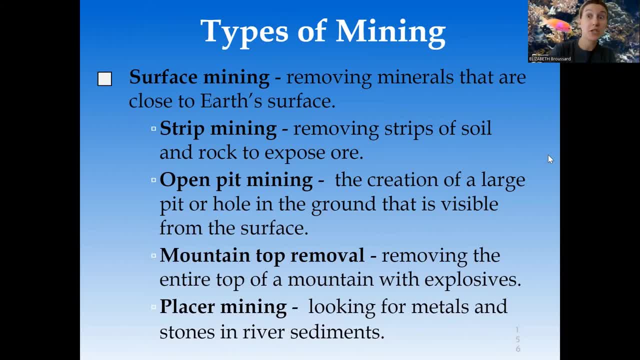 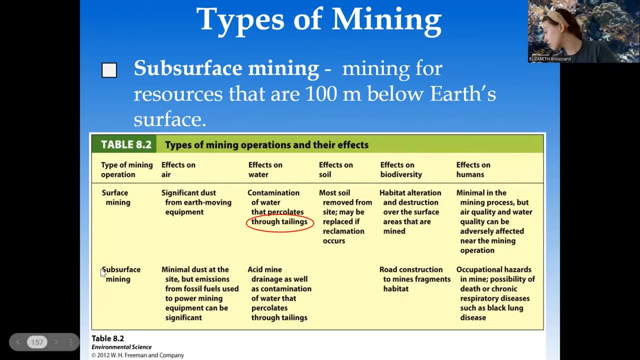 We will also talk about mining more in class when we mine for chocolate chips. Our subsurface mining is also goes over. it's reviewed in that page 227 on in your textbook. But our One and only type of subsurface mining: instead of exposing by digging a hole or exposing things at the surface like in surface mining, in subsurface mining. 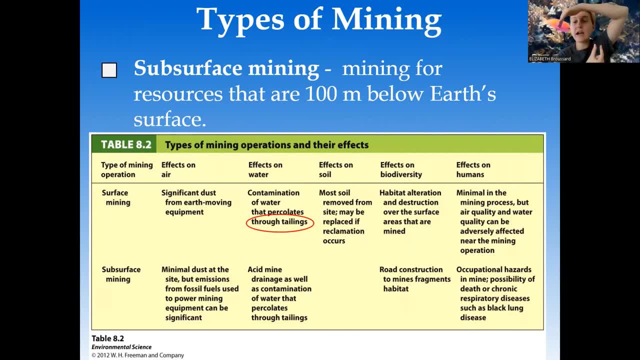 I'm looking at the mountain and I'm actually just going to dig a skinny, tiny horizontal- excuse me- vertical tunnel and then I'm going to mine. in that way, While subsurface mining can be a more intensive process- and it's going to be- obviously it's much easier to just get some dynamite and like, blow things up and like just 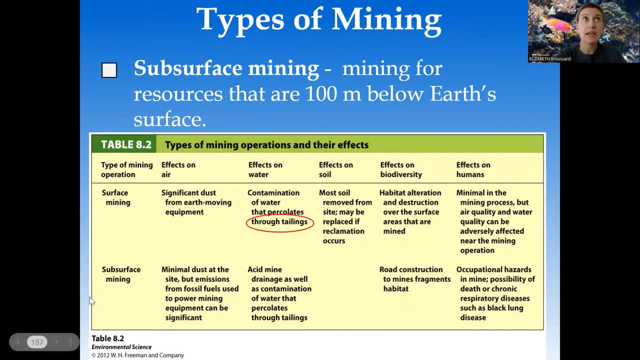 get to it. that way, Our subsurface mining is going to end up being the most environmentally friendly, Because one thing that you have to worry about, whether you're doing surface mining or subsurface mining, is something I've circled here known as tailings. 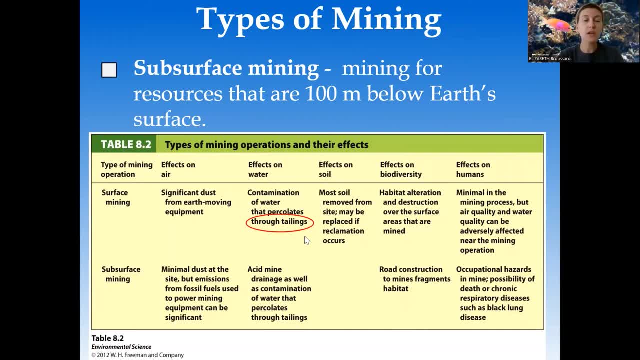 Tailings is going to be the debris, the rock debris that results from mining processes. So the more explosive you are, the more tailings you're going to have, and sometimes these tailings can be detrimental for ecosystems by. take some Dean TNT, Blow up a mountain and then I have debris everywhere. that debris, when it rains, is going to trickle down into my streams, is going to affect my aquatic ecosystems. 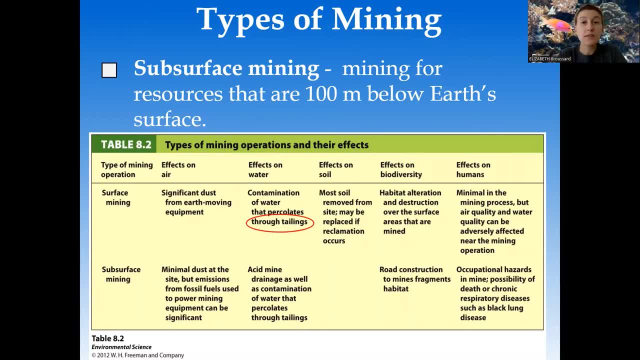 It can then be found into the soils and just kind of cause a lot of detriments in total, which is kind of summarized by this: effects. So our subsurface mining ends up reducing the amount of tailings, reducing the amount because of just doing that narrow hole. 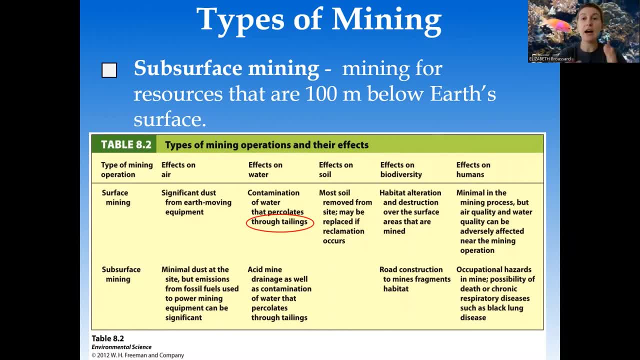 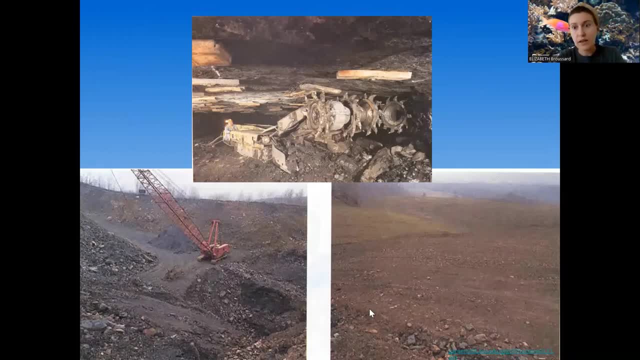 I wish that you guys could see the picture. please go to page 227.. We'll talk about all that. Here's some pictures again showing we can see if there's a lot of debris. There's a lot of. I'm in. some of this stuff is just super fine dust.